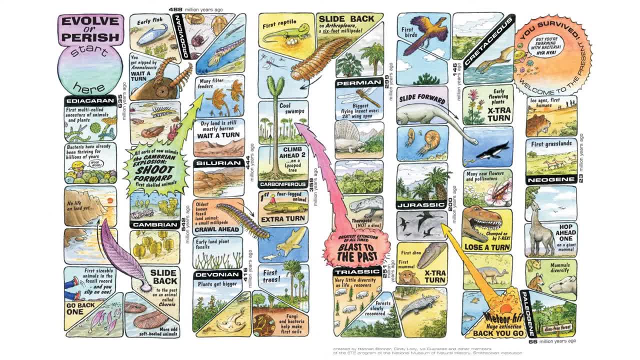 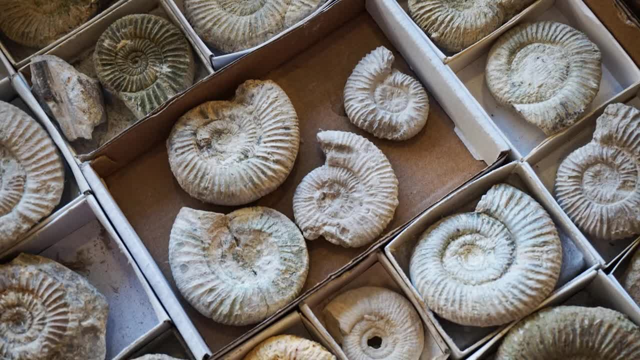 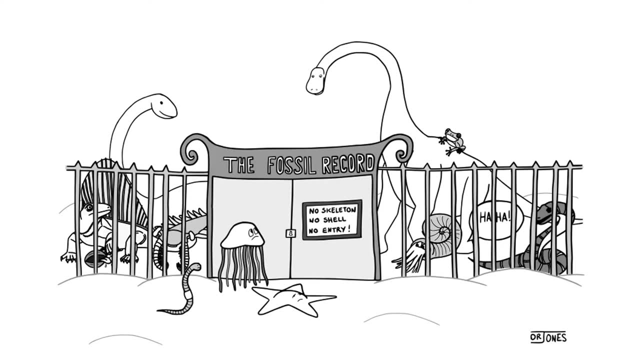 What major evolutionary events were necessary to create the world. we have now To address these questions and others. paleontologists study the fossil record, But we know that the fossil record isn't perfect. In fact, it's actually incomplete. Many species are missing. it primarily consists of hard parts and the vast majority of fossils. 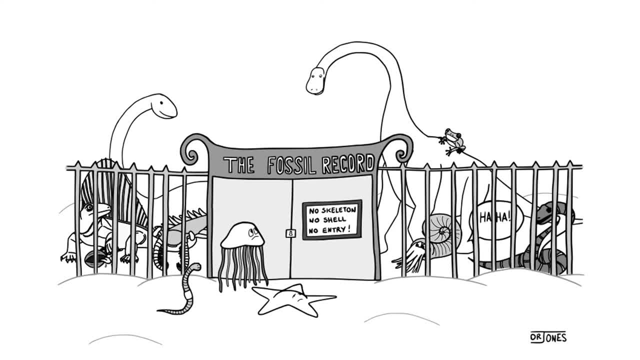 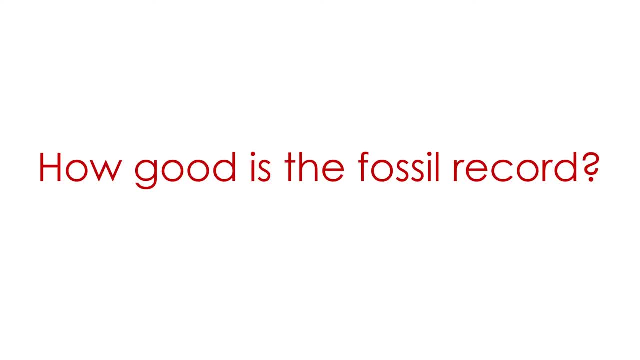 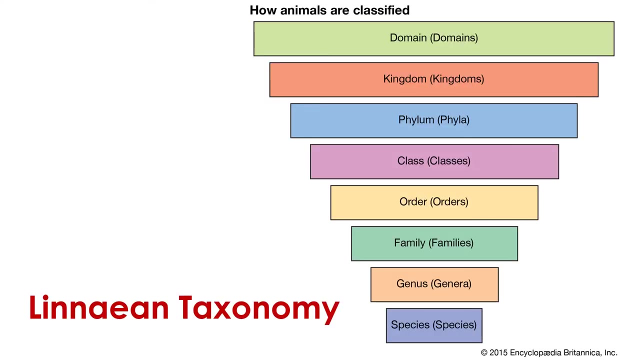 get destroyed before paleontologists can collect and study them. This begs the question: how good is the fossil record? How well does it capture the history of life And what organisms left behind the most fossils? These are the main questions. Recall that we use a classification system called Linnaean taxonomy to name and group. 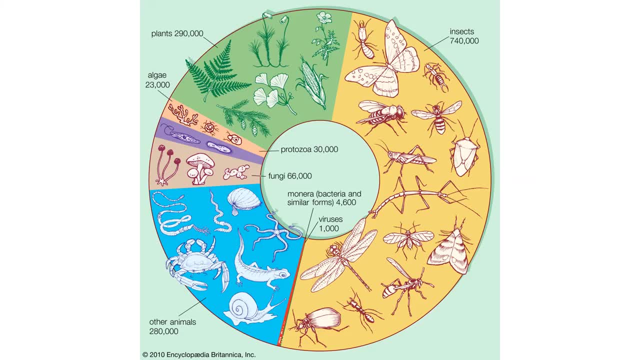 taxa together. Using this system, scientists have identified more than 1.4 million species on our planet today. Of these species, over half are insects, About one quarter are insects, other animals and the rest are plants, fungi and prokaryotes. paleontologists in 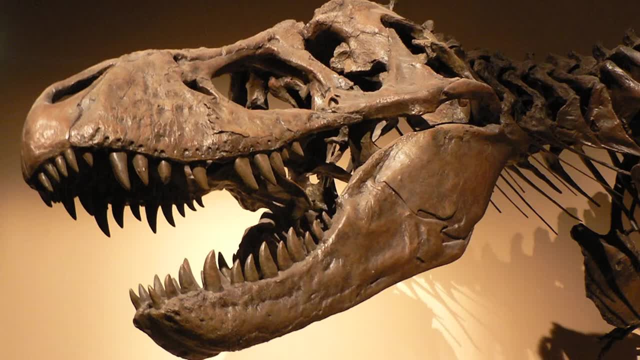 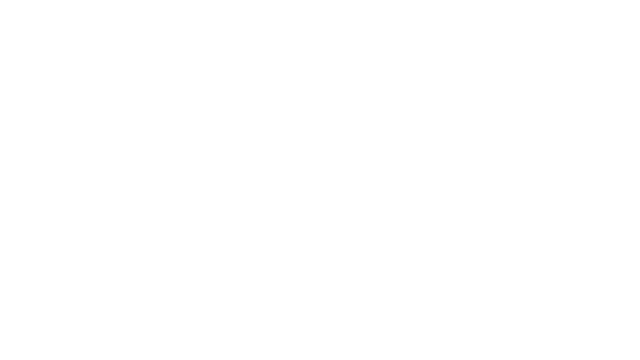 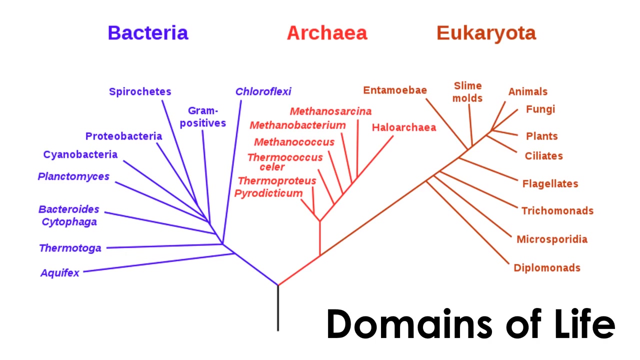 contrast, have only discovered around 250,000 species in the fossil record thus far. the number keeps growing, but we can be certain that far more than 250,000 species existed on our planet in the past. if we break the fossil record down by tax on, we find that the record has other issues too. generally speaking, all. 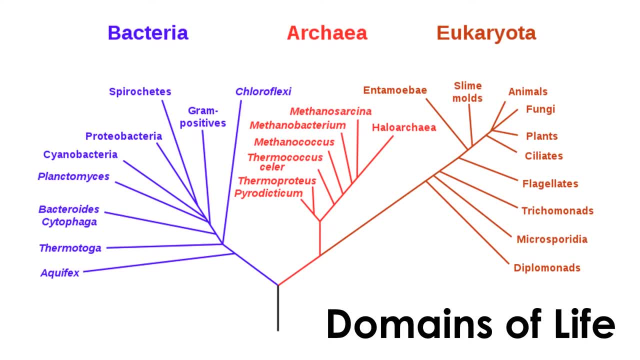 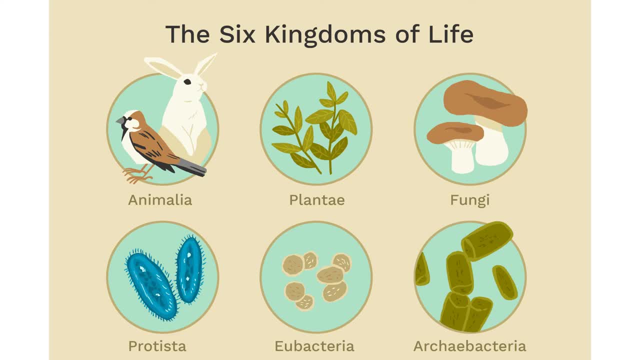 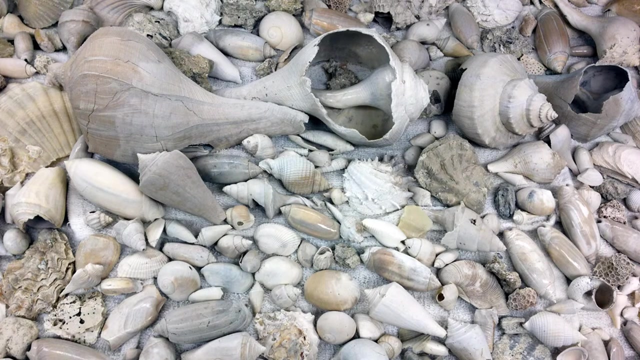 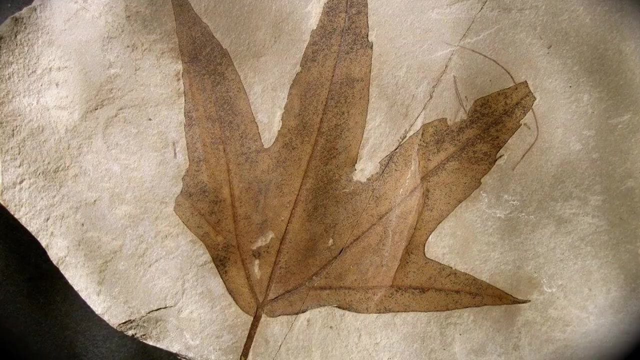 three domains of life are probably represented by fossils. however, the vast majority of fossils come from just three kingdoms: animalia, plantae and protista. there are very few fossils of fungi. if we look further at the record, we find that most fossils come from animals. fossils of 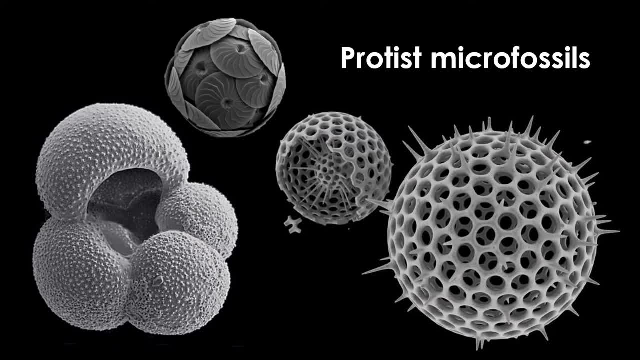 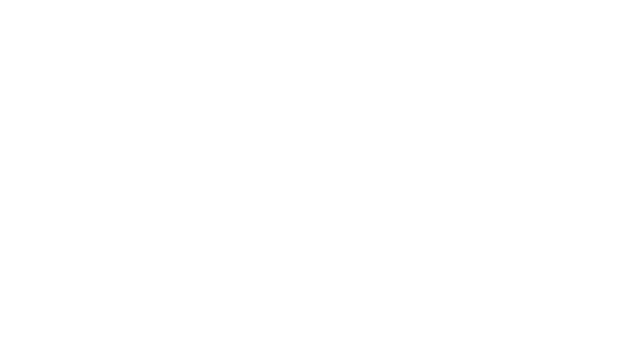 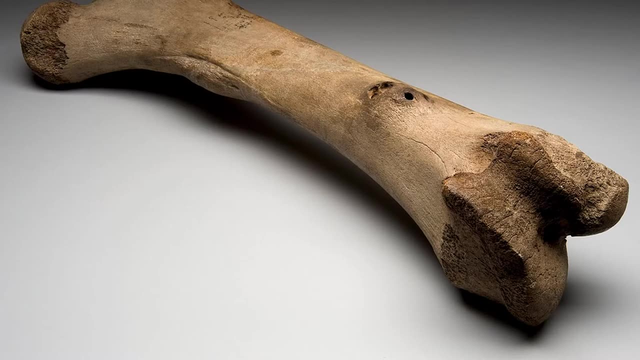 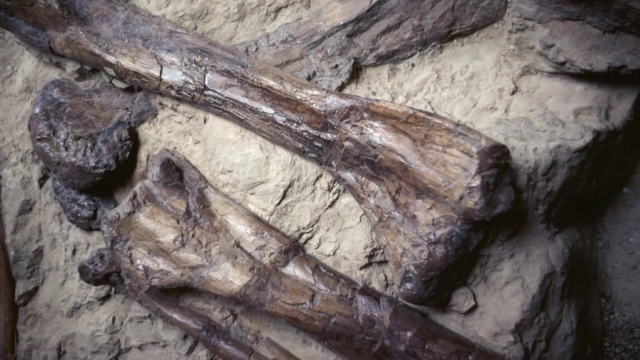 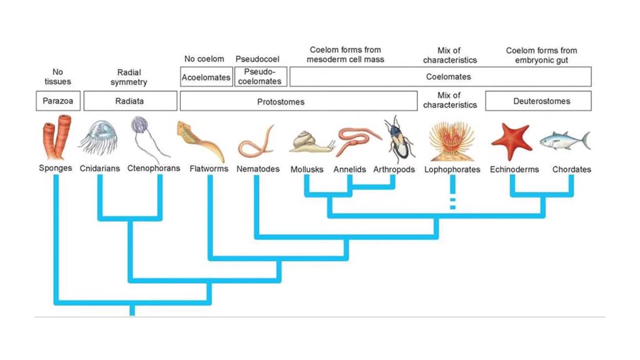 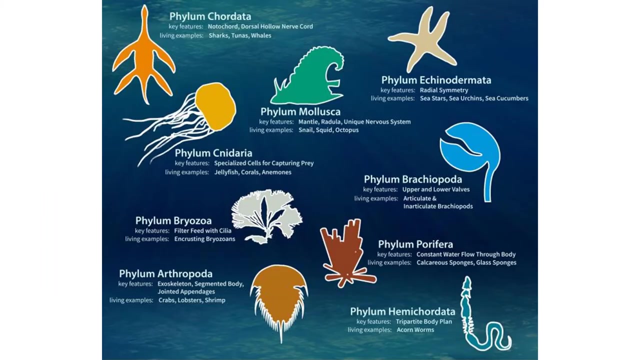 plants and protists are not uncommon, but animals are by far the most abundant. why is this the case? animals produce large hard parts like bones, shells and teeth, which stand a much better chance of being fossilized than pieces of plants or protists. overall, the animal kingdom includes over 35 phyla, but if we look very closely at the 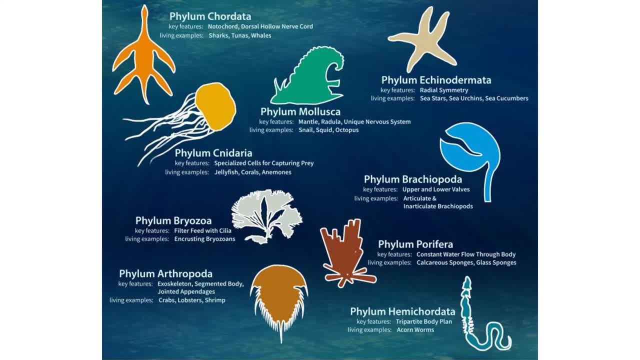 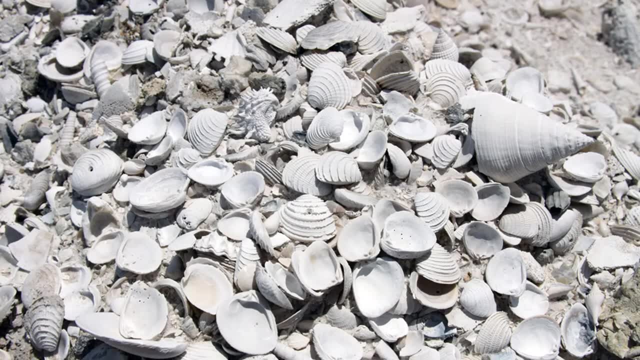 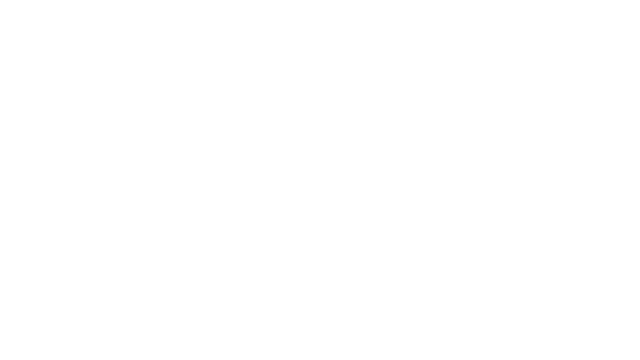 fossil record, we see that the vast majority of fossils in the world are vast vast majority of fossils come from just nine of those 35 phyla. again, the reason is simple. these nine phyla produce hard body parts that stand the best chance of becoming fossilized. so what are the nine animal phyla that make 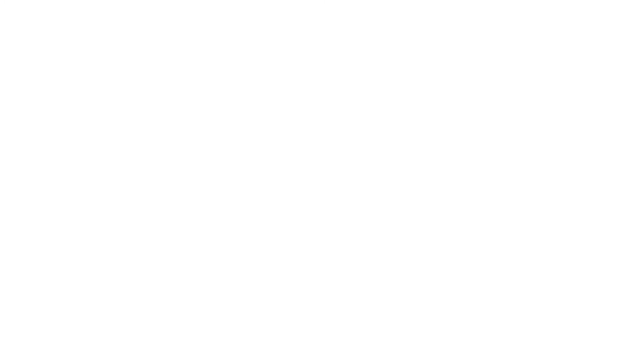 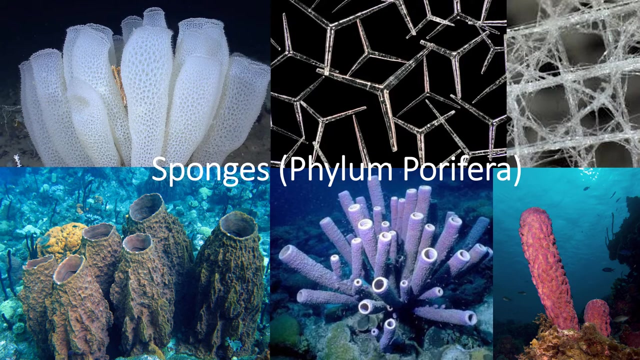 up the bulk of the fossil record. porifera is the name of a fossil record, the name of the phylum of sponges. sponges are the simplest animals and we're probably the first animals to originate on earth. they do not have true tissues, so they don't have nervous, digestive or circulatory systems. their 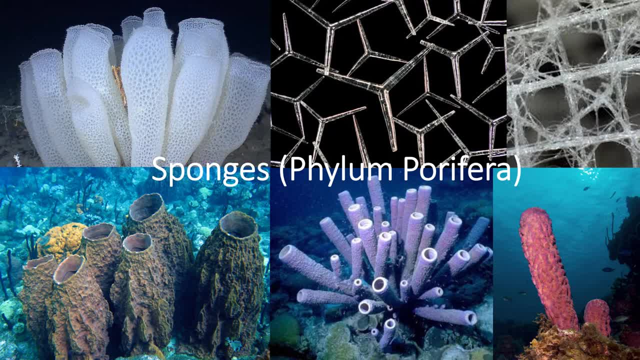 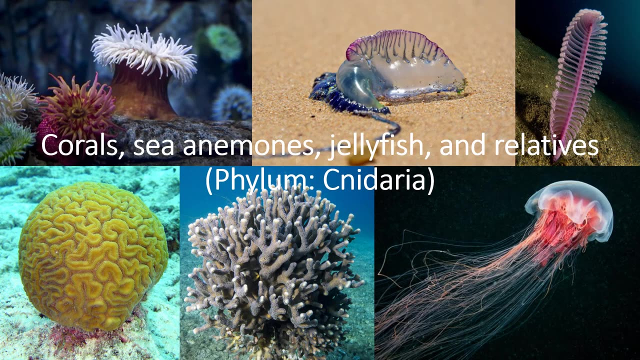 bodies consist of only two layers of cells, but with the exception of bath sponges, these animals produce skeletons made of silica and calcium carbonate, which are sometimes preserved as fossils. phylum nidaria includes corals, sea anemones, jellyfish and their various relatives, jellyfish, sea anemones and the. 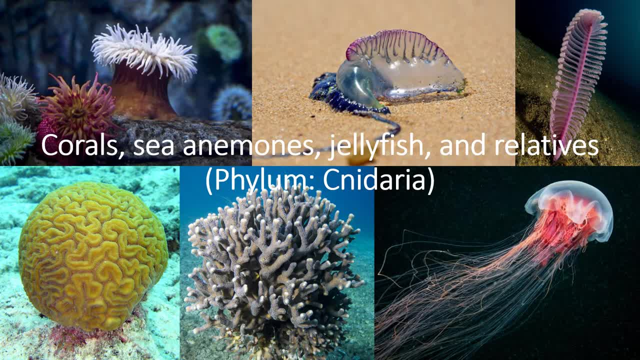 rest have a very poor fossil record, but coral fossils are quite common in rocks of phanerozoic age. this is because corals are heavy biomineralizers. they produce massive skeletons made of calcium carbonate. these skeletons are the foundations of coral reefs you may not have heard of. 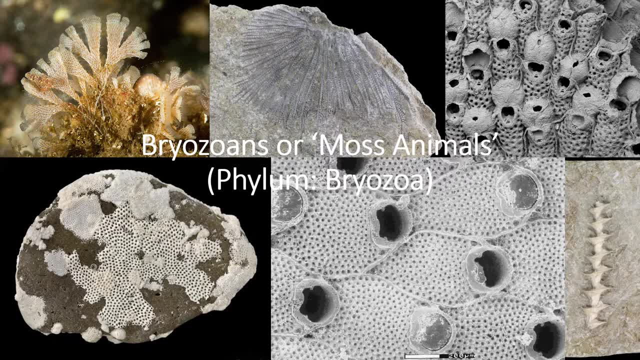 bryozoans and if you saw one you would probably call it a coral. but the phylum bryozoa is very diverse. in the fossil record, bryozoans are most common, known as moss animals, because they grow on many structures by encrusting them. 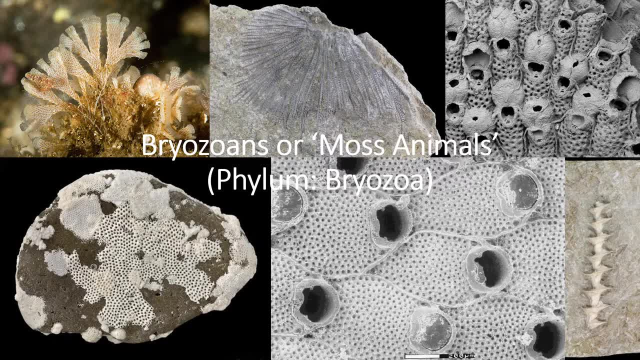 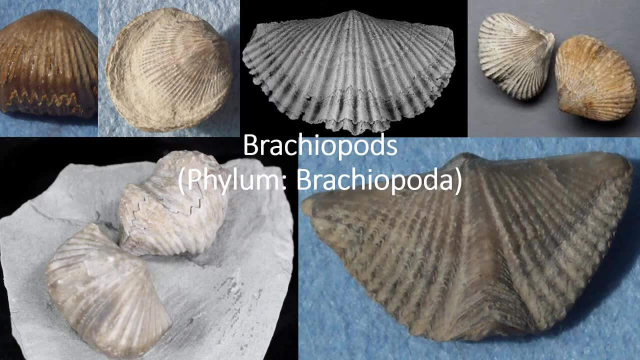 like moss, but unlike moss, and like corals, bryozoans produce robust skeletons made of calcium carbonate. brachiopods look a lot like clams, but they are actually more closely related to the moss animals. species in the phylum brachiopoda produce bivalved shells made of calcium. 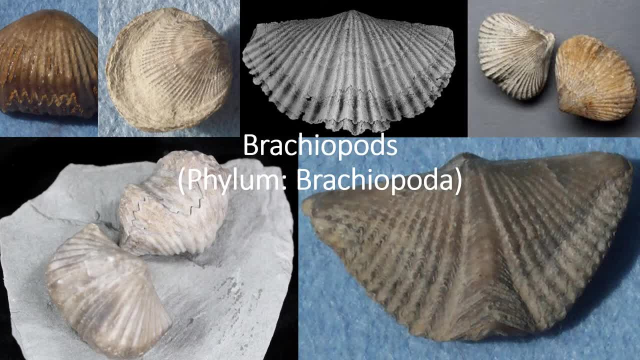 carbonate and calcium phosphate. today, brachiopods are somewhat uncommon. you only find them in low-energy lagoons and other restricted environments. but during the Paleozoic era, between 541 and 252 million years ago, brachiopods were some of the most common animals that lived in the phylum brachiopoda. the most common animals. 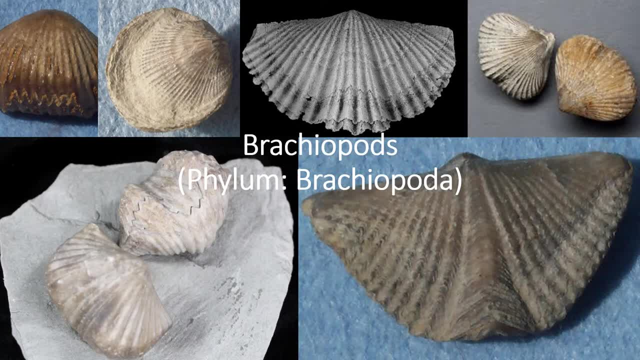 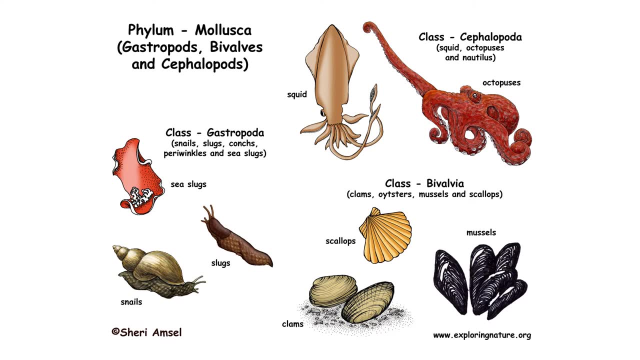 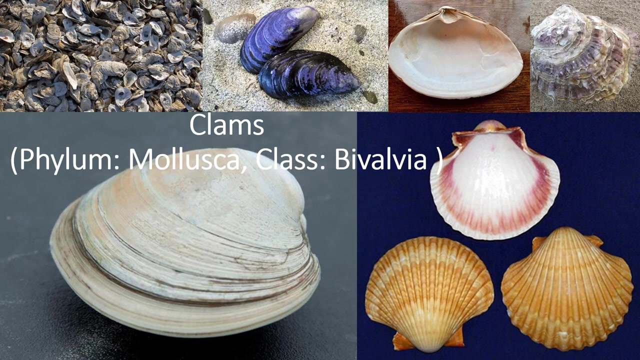 in most marine environments. the phylum mollusca includes a wide array of different animals, including clams, snails, squid and octopi, in addition to many other taxa, clams belong to the class bivalvia in the phylum mollusca. their shells consists of calcium carbonate in the form of the bivalve shell with a 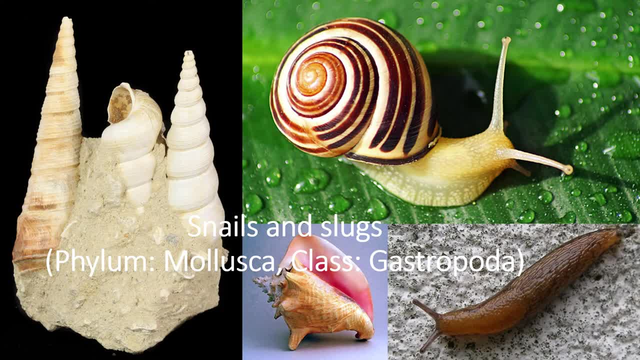 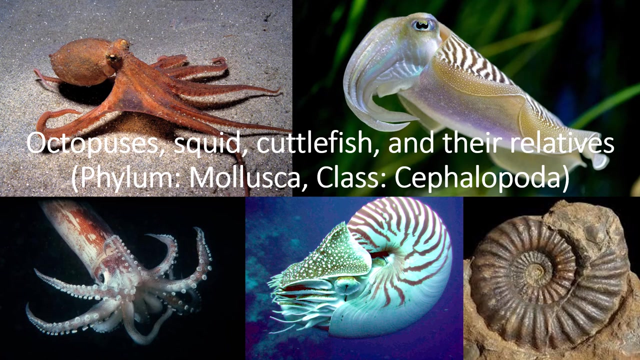 mineral aragonite. snails and slugs make up the class gastropoda in the phylum mollusca. snails have a great fossil record because, like clams, they produce shells made of aragonite. squid, octopi and cuttlefish belong to the class. 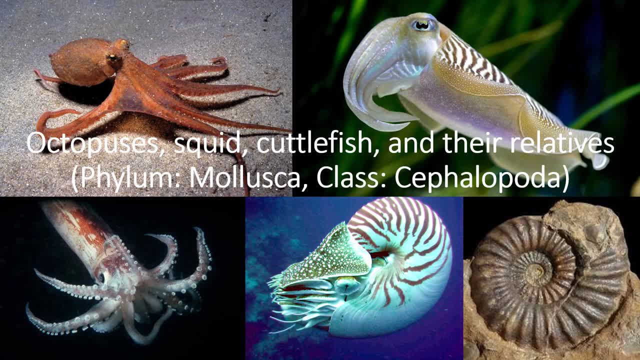 cephalopoda in mollusca. unlike other molluscs, these creatures obviously don't have hard shells and for this reason there are generally very few fossils of these animals in the fossil record. nonetheless, there are a number of extinct groups of cephalopods, like ammonites, which did produce massive 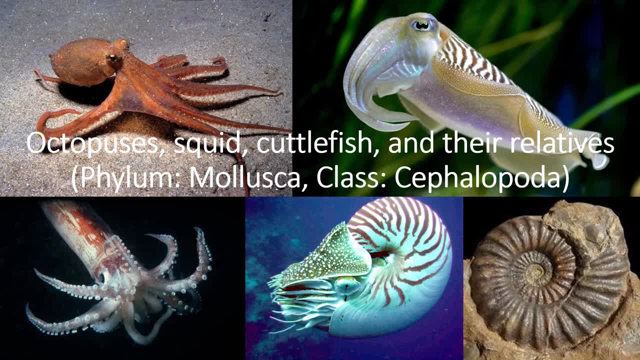 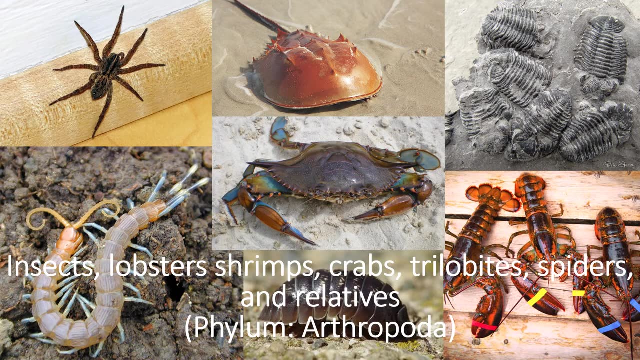 shells made of aragonite. although these groups were not found in the fossil record, they were found in the fossil record in the. the phylum arthropoda includes animals with segmented exoskeletons which they frequently molt. they include lobsters, insects, shrimp crabs, spiders, horseshoe crabs and other similar creatures. they 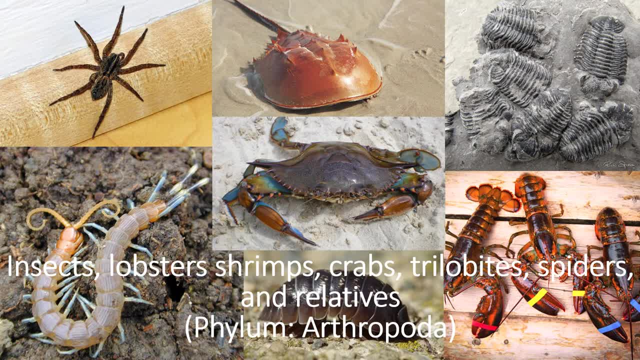 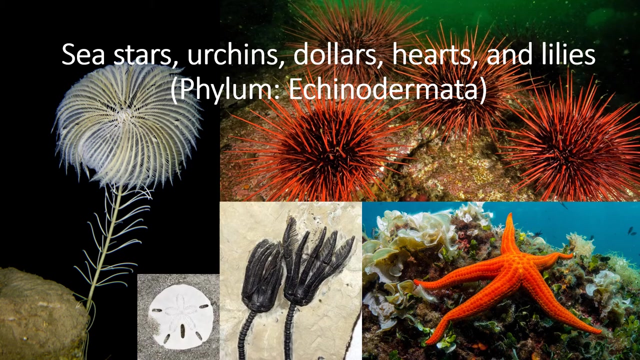 also include trilobites, which went extinct 250 million years ago. trilobites are the most diverse group of animals in the fossil record that is now extinct. trilobites produce thick exoskeletons made of calcium carbonate minerals. echinoderms include starfish, sea urchins, sand dollars, sea lilies and sea cucumbers. 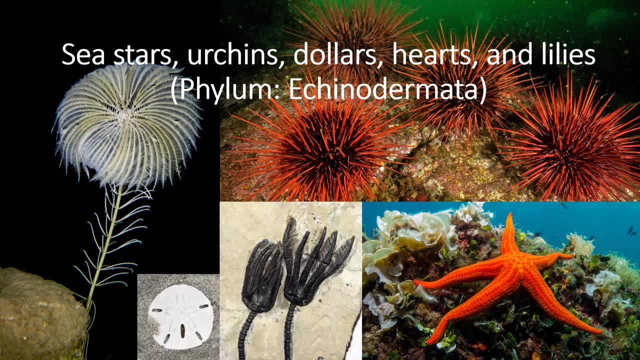 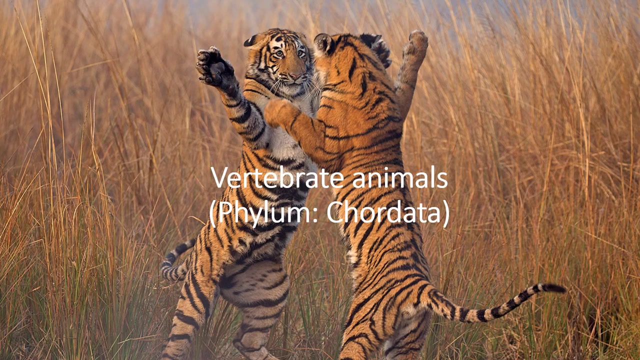 there were also a number of major groups of echinoderms in the paleozoic era which are now extinct, with the exception of sea cucumbers. echinoderms produce mineralized skeletons made of calcium carbonate. this makes them highly preservable as fossils. the phylum cordata includes all animals with 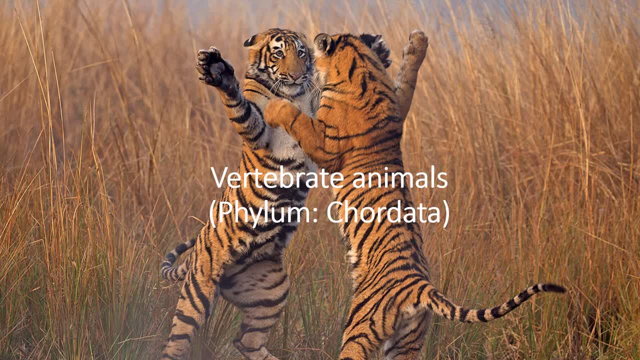 vertebrae, backbones and jaws. the phylum cordata includes all animals with vertebrae, backbones and jaws. the phylum cordata includes all animals with vertebrae, backbones and jaws: sharks and rays, fish, amphibians, snakes, turtles, reptiles, dinosaurs, birds and. 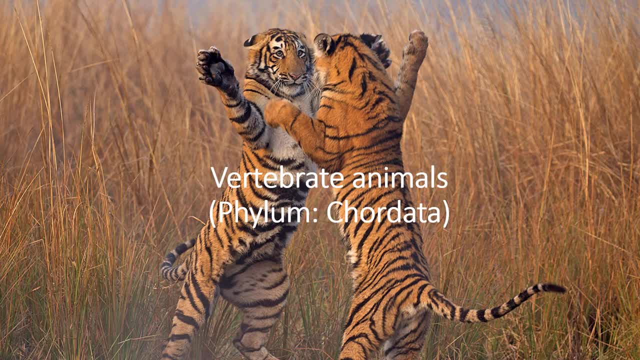 mammals. they all belong to this phylum, with the exception of sharks and rays. these animals all produce skeletons, bones and teeth made of calcium phosphate in the form of appetite minerals. finally, a better example is an anhydrite that is made of calcium phosphate and later used for food and medical use. 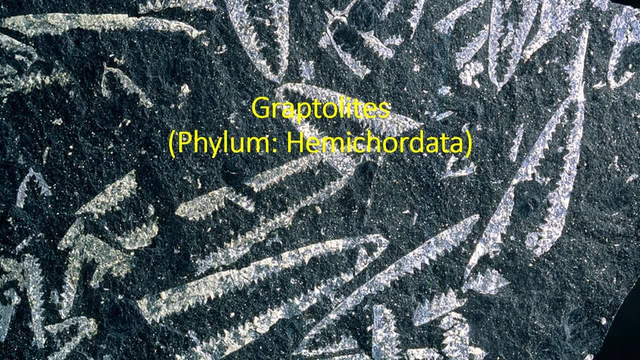 Finally, the last major phylum in the fossil record is the phylum Hemicordata. Most Hemicordates in the fossil record are called Graphtolites. Graphtolites are now extinct, but they were very common in the early Paleozoic, when they